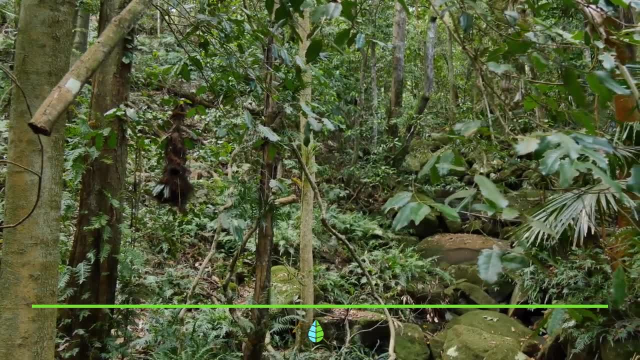 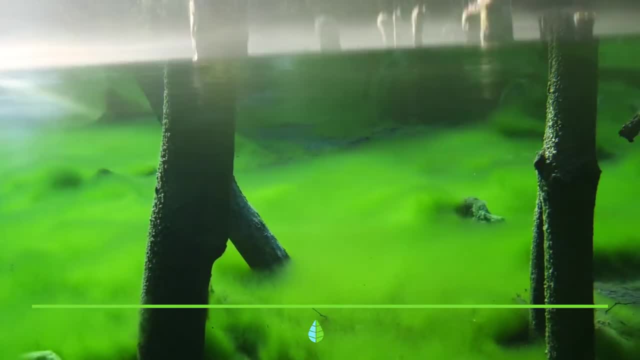 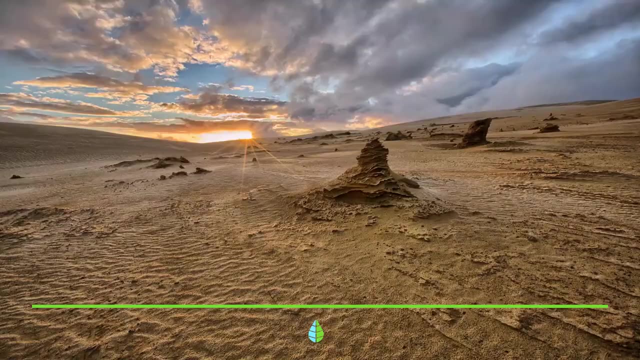 birds and other animals. We can classify ecosystem between natural and artificial, but only natural ecosystems have more subtypes. Therefore, in this video, we'll be talking about the four types of ecosystems: terrestrial, aquatic, mixed and artificial Terrestrial ecosystems. Terrestrial ecosystems are those in 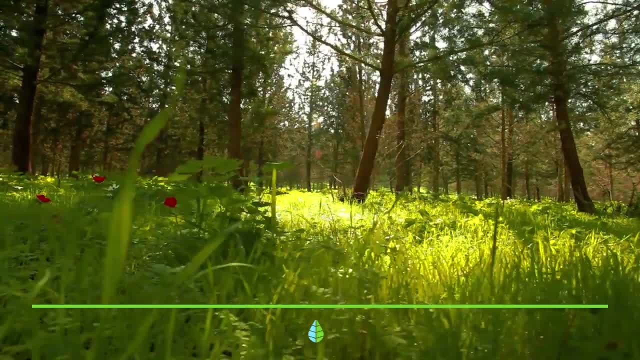 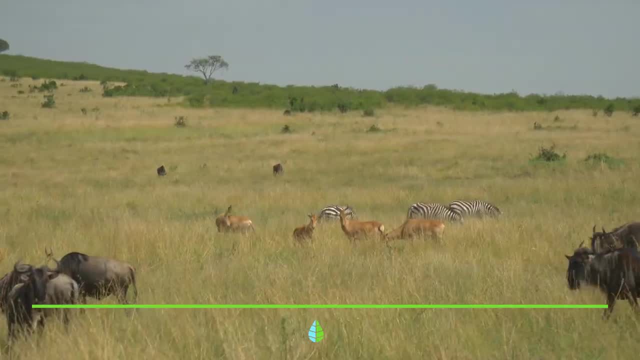 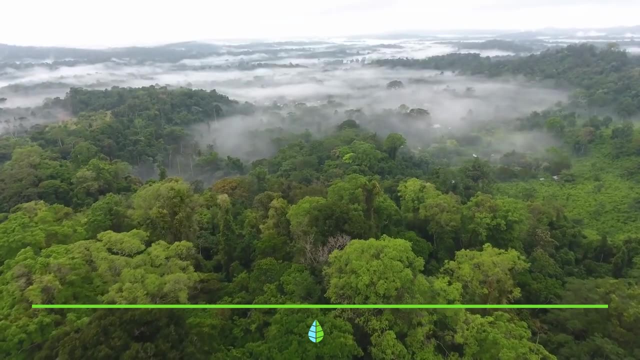 which living beings inhabit the soil or underground in. This ecosystem occupies 30% of the world's territory and is divided into the following types: Deserts, which occupy 30% of terrestrial ecosystems. Savannas and tropical grasslands, which occupy 20% of terrestrial ecosystems. Jungles, occupying 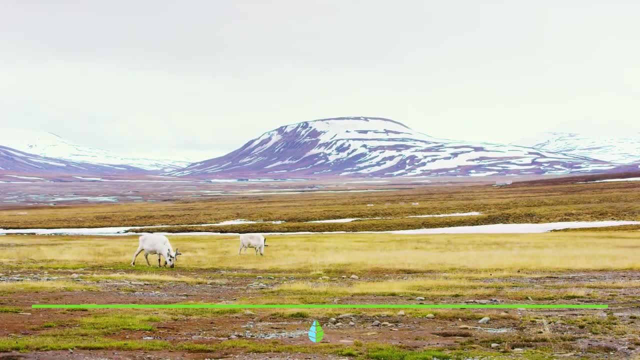 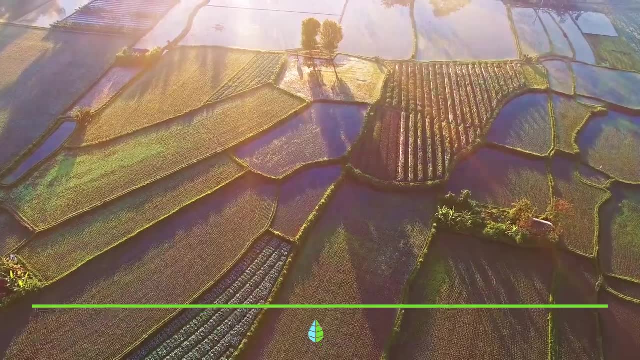 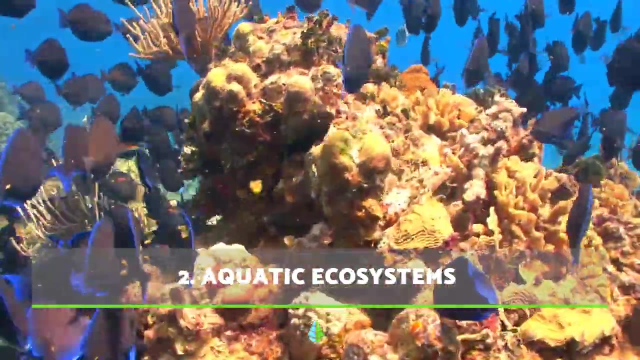 23%, Temperate forests and tundras occupying 17%. And finally, among the terrestrial ecosystems, there are also the cultivators. The cultivators are the ones that occupy the 10% of the world's territory. Aquatic ecosystems: Aquatic ecosystems are characterized by the presence of water. 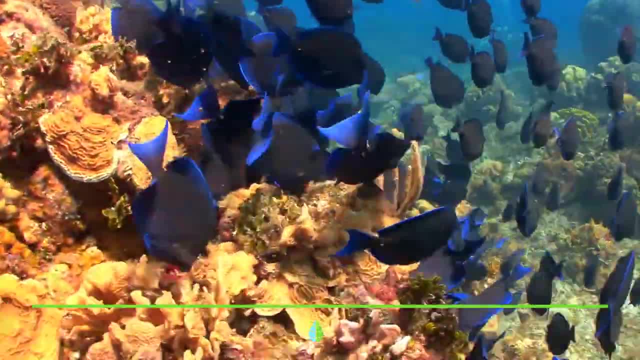 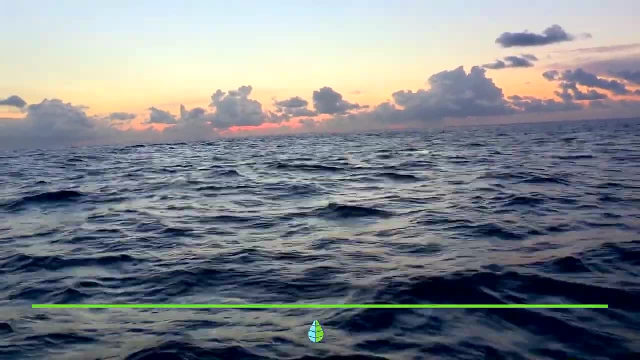 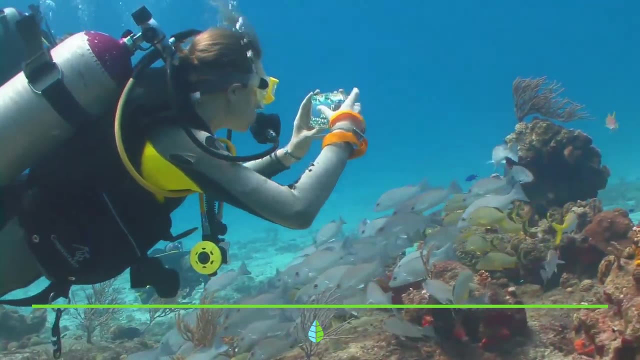 as the main physical component. This water can be sweet or salty, So we find two types of aquatic ecosystems: Marine ecosystems: These include all saltwater ecosystems such as oceans, seas, reefs, shallow coastal waters, etc. And freshwater ecosystems, including lakes, ponds, rivers, streams and. 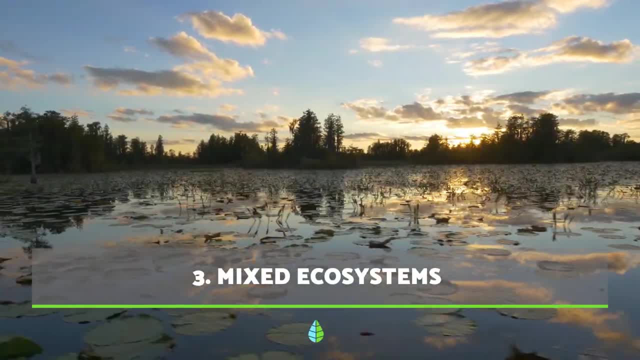 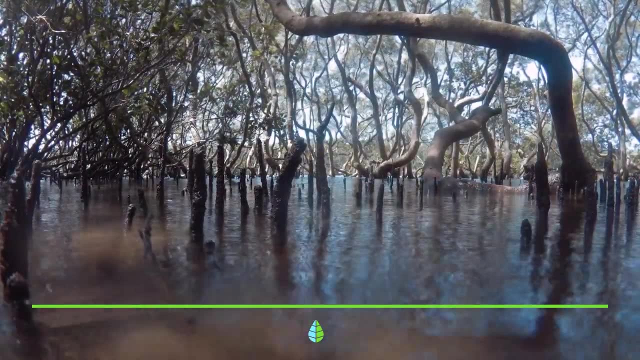 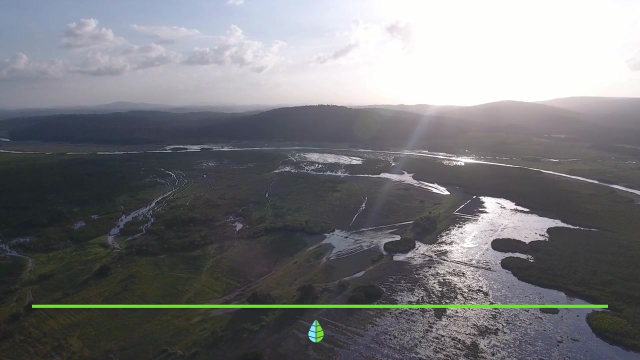 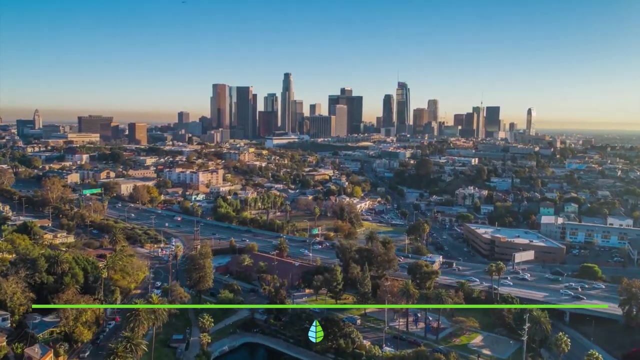 springs. Mixed ecosystems. Mixed ecosystems are those that are located between two different types of terrains, For example water and earth. The main types of mixed ecosystems are wetlands, mangroves, marshes and coasts. Artificial ecosystems. Artificial ecosystems are unnatural ecosystems created or changed. 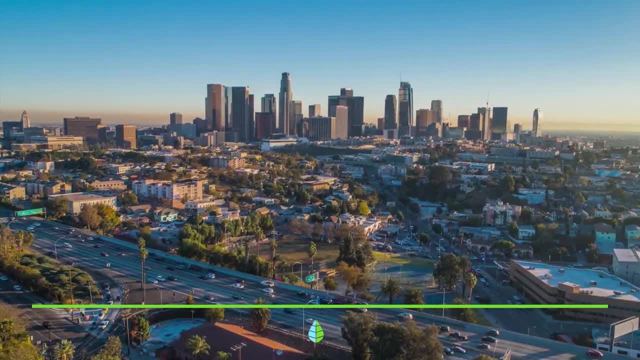 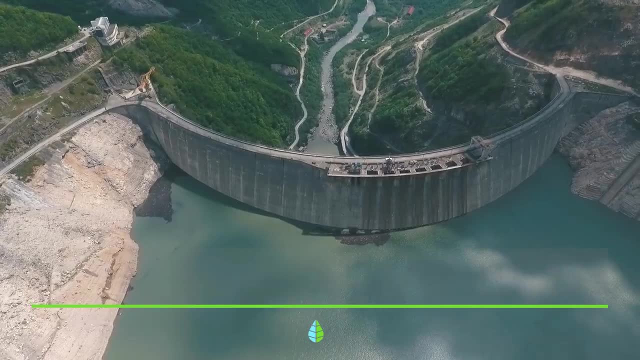 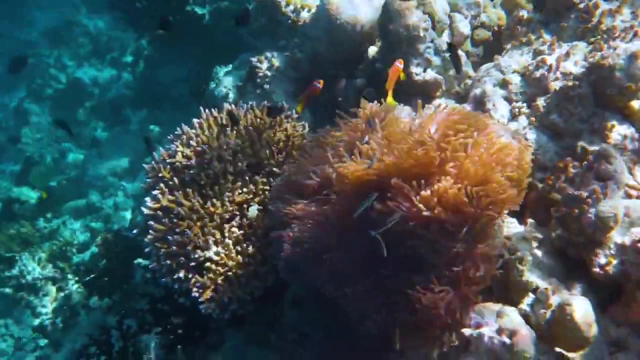 by humans. The main types of artificial ecosystems are urban ecosystems, agricultural ecosystems or reservoir ecosystems- The living beings of an ecosystem. Each ecosystem has a great variety of living beings that form part of that system. Each of them have different functions in the balance of that ecosystem. This